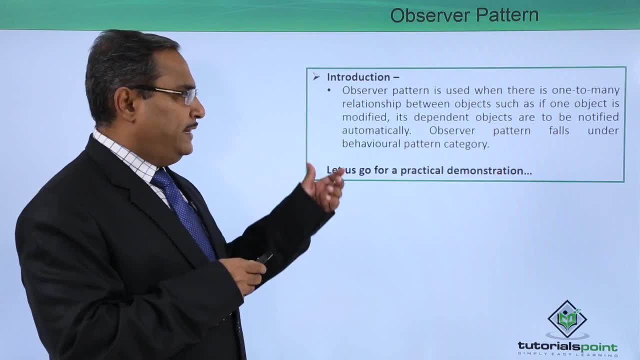 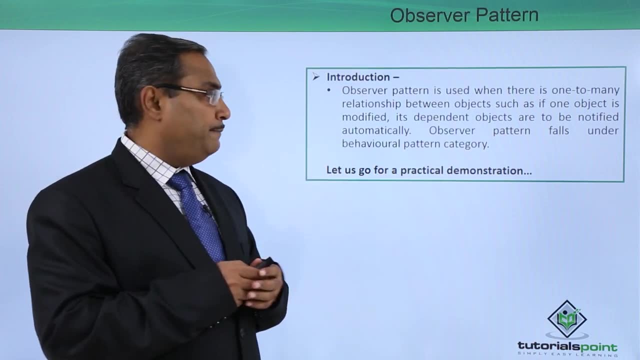 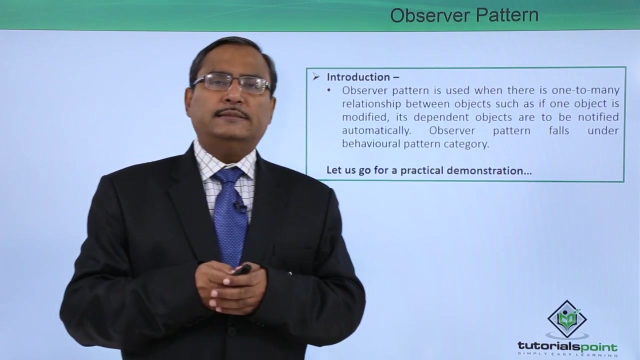 the cardinality ratio will be there. In that case, if the one object is modified, its dependent objects will get the notification automatically. Observer design pattern falls under the behavioral design pattern category, So let us go for one practical example using Java and also. 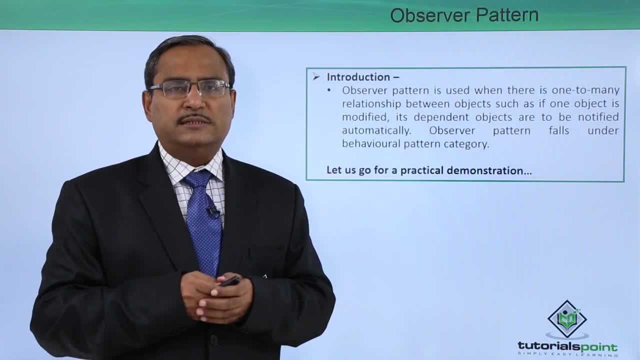 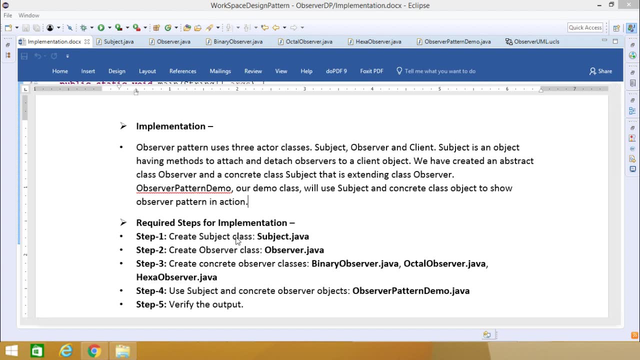 email class diagram for the better understanding on this concept. So here is the demonstration for you. To understand observer pattern, first we need to understand the subject and the observer objects. The relation between the subject and the observer can easily be understood as an analogy to, say, online course subscription, An online course publisher also known as the. 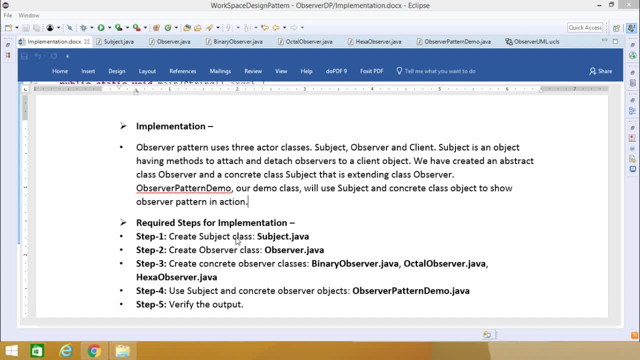 subject is in the business and publishes courses, we can consider them as data. If we- that is, the user of data or observer- are interested in the course, So we subscribe. that means we register, and if a new edition is published it gets delivered. 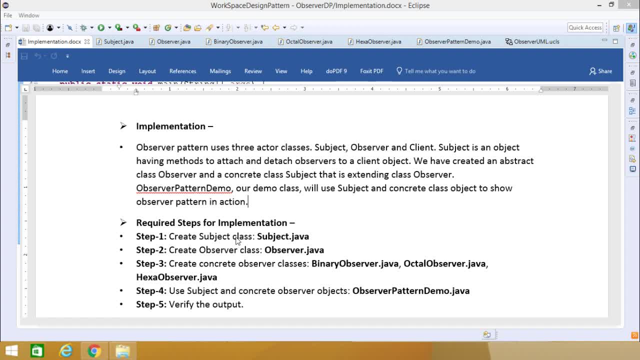 to us and if we unsubscribe- that is unregister- we stop getting new editions and publisher does not know who we are and how we use the course and it just delivers it to us because we are a subscriber, and it is also known as loose coupling. So now let us go for the 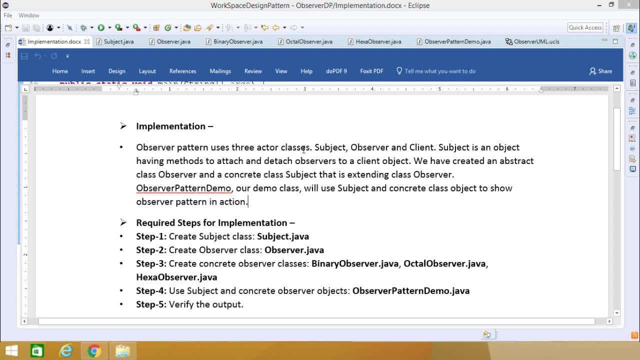 implementation. So observer pattern uses 3 actor classes, subject, observer and client. So subject is an object having methods to attach and detach observers to a client. object We have created an abstract class observer and a concrete class subject, and that is extending. 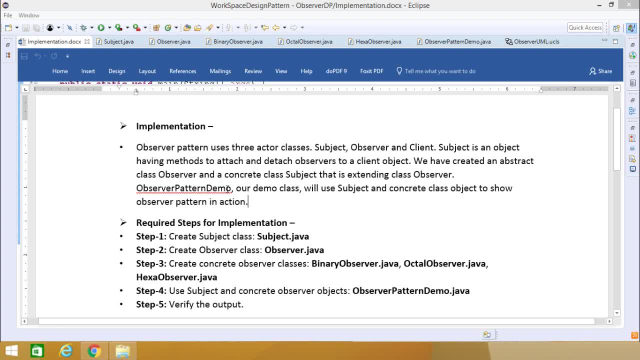 class observer, So observer pattern demo. our demo class will use subject and concrete class object, show the observer pattern in action. so let us discuss them through the codes and step by step. so request step for the implementation will be step one. so create subject class that is a. 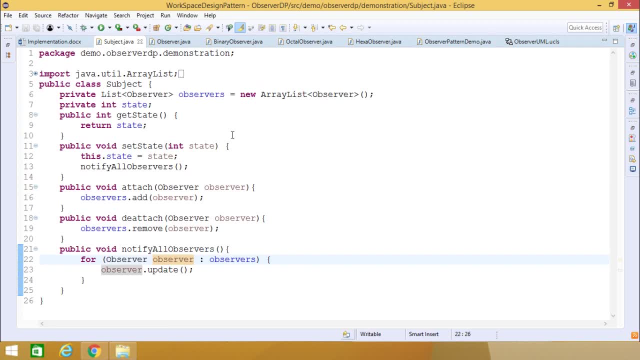 subjectjava. so here you are having this code. here there is a subjectjava, so public class subject, and it is having one uh: observers, that is the array list which can hold observer objects. we're having int state, we're having this get state which returns state, so it 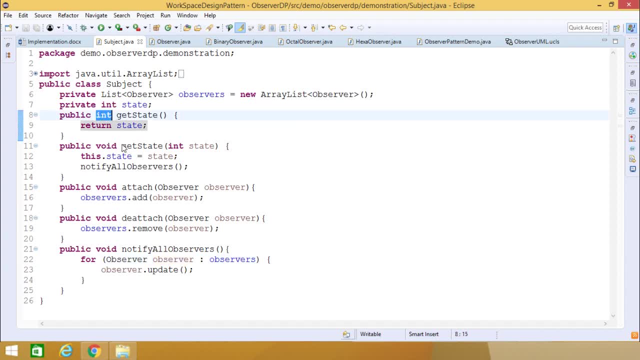 having the output argument, that is the int. we're having the set test say state. we're having this int state as input argument and this dot state is equal to state. so that will be assigned and notify all observers. so this particular method will be called in case of set state. now, public void attach. 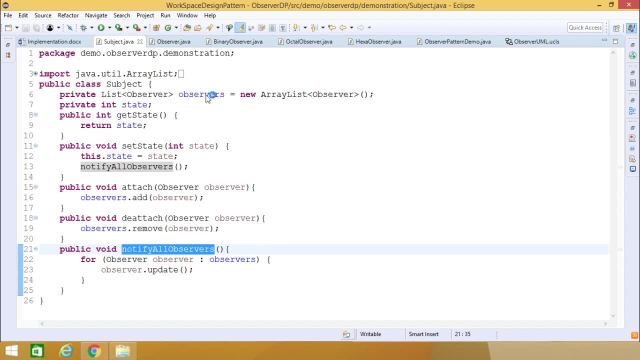 so where this observer object will be passed and this object observers this array list will will have the this addition of this new observer object. in case of detest, we'll be using the method remove observers dot remove and in our notify all observers we use this for each loop. so observer, observer colon observers and observers dot update. so in this way, 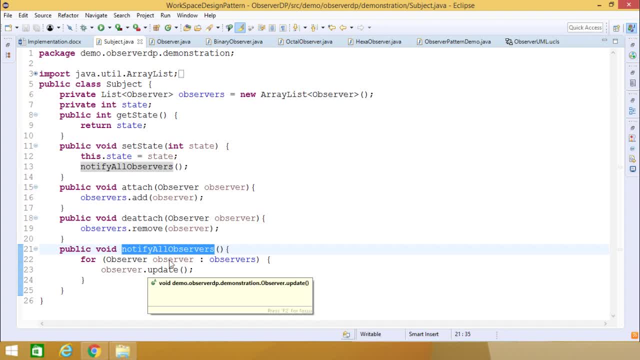 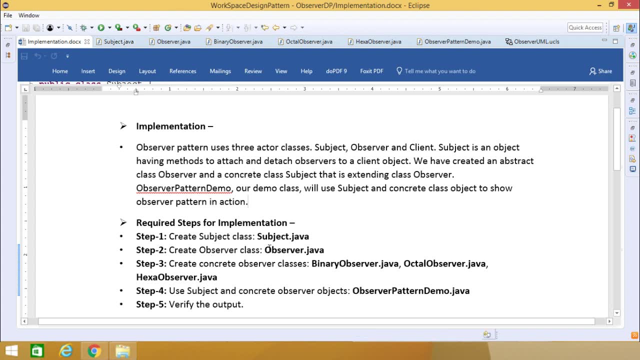 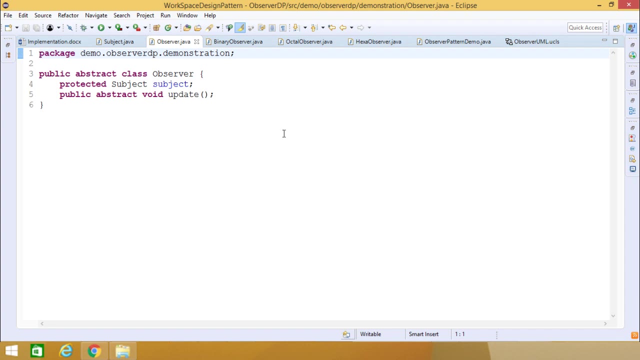 we are having this, so observers dot update this method. we have written under this observer dot Java, so now we are going for the second step, that is, the create observer class, that is, observer dot Java. so here we are having this observer dot Java, so protected subject. subject: public abstract void. 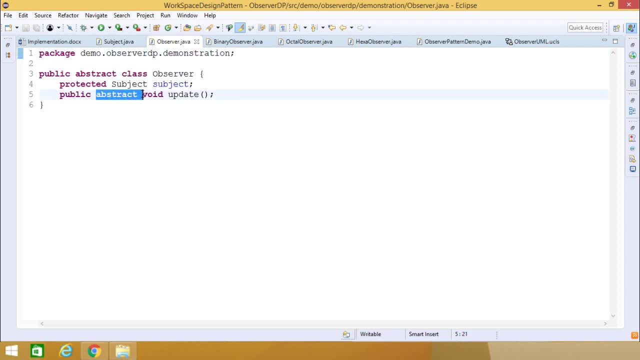 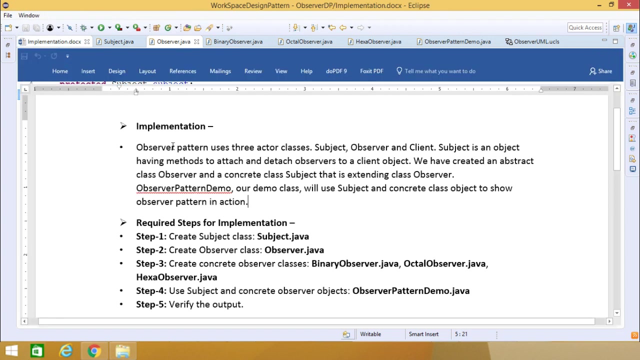 update. so, as it is, the method is of the type abstract, so its body has not been written here and also the class has been called as abstract class observer. so we have discussed this subject- dot Java- and also we have discussed this observer dot Java. now we are going for create concrete observer classes. 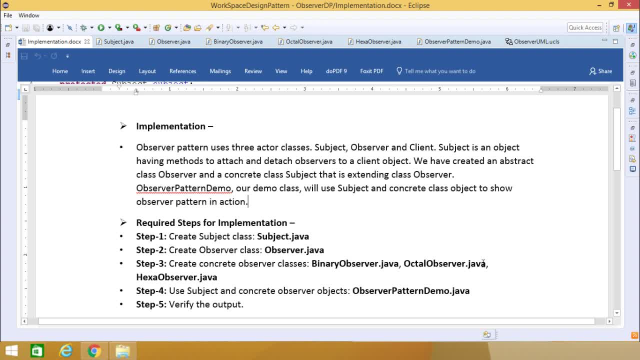 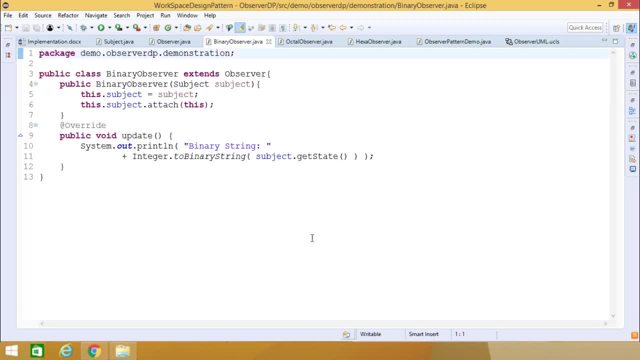 and there is a binary observer, dot Java, octal observer, dot Java and hexa observer, dot Java. so now this is our binary observer, dot Java. so in this particular class we are having this binary observer, that is a constructor which will take the subject, and this dot subject is equal to subject. 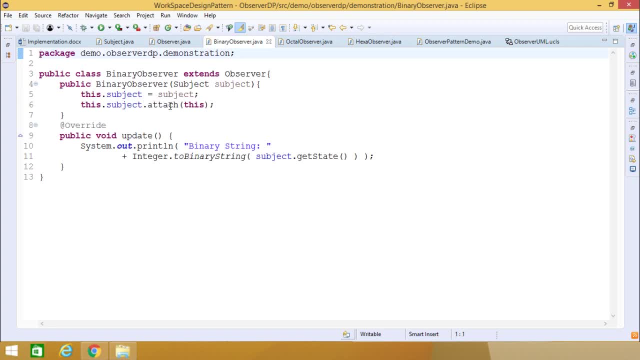 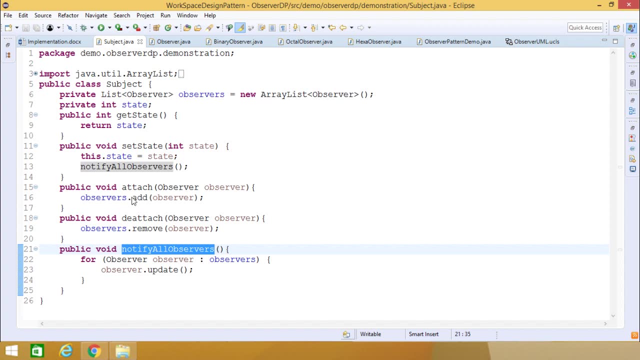 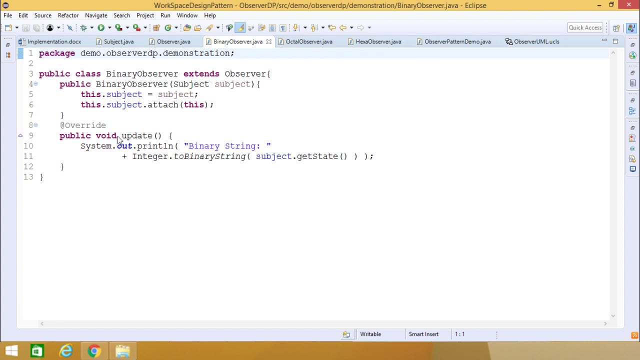 dot attached this. so now what will happen? this is a subject and this is the attach function which will issue this: add a list, dot add, so observers, dot add so. in this way it will get added with the add a list, and here we are supposed to implement the update function. so update method is there, which. 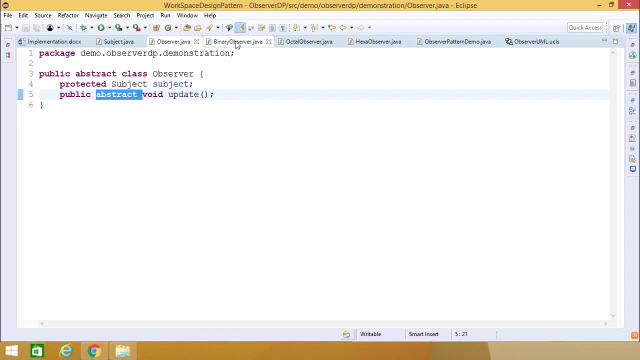 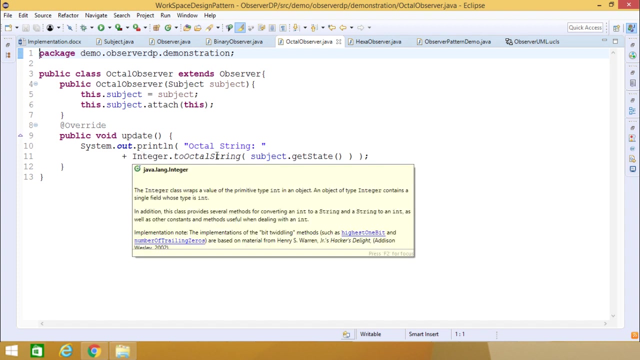 was there. in the abstract class, abstract method update, we have written the respective body. so here we have an integer dot two binary string. we are getting this in case of octal observation of observer. we have done the same, but here we have written integer dot two octal string. so you can. 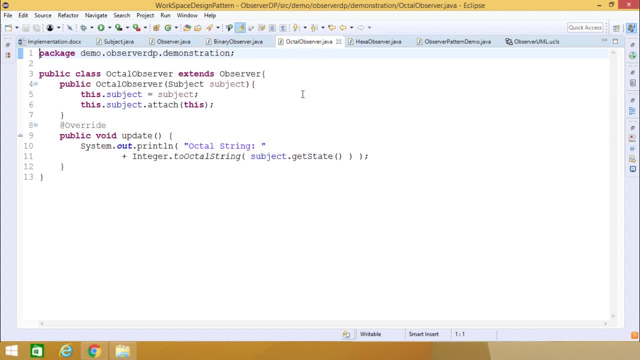 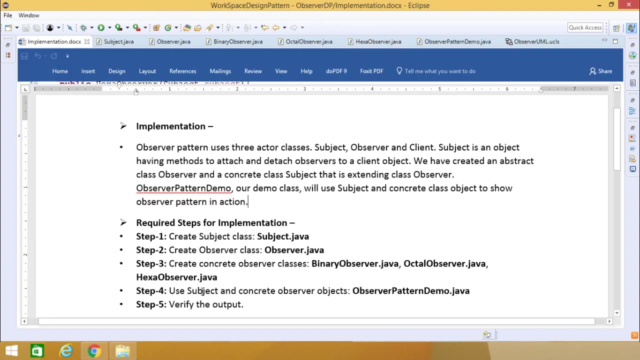 find that binary observer dot Java, octal observer dot Java, that also having the same code, same type of code, we're having hexa observer dot Java, which is also having the same type of code. now we are going for implementation dot Docs. so that is step number four. use the subject and concrete observer objects. observer pattern demojava. 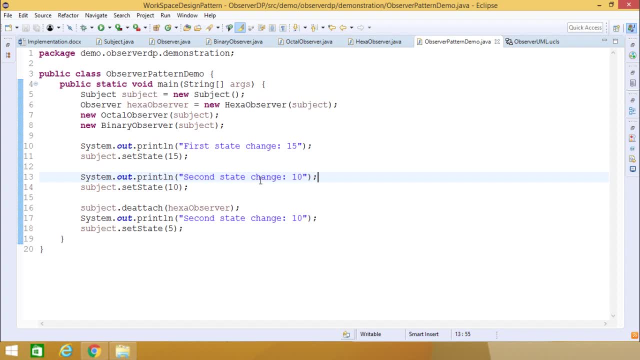 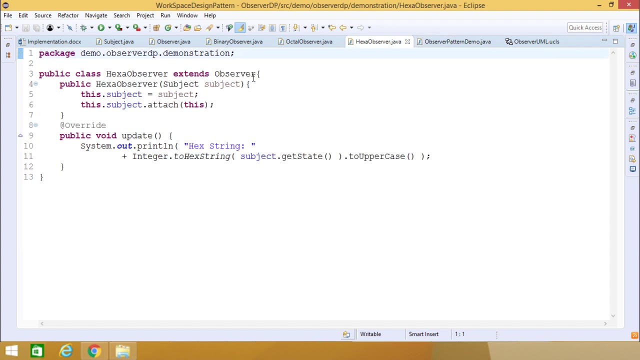 so this is our observer pattern demojava. here you can find that here we have defined one subject object, and then we are having this observer. hexa observer is equal to new hex observer subject. so now you can find that whenever we are calling this constructor, whenever we are calling this, 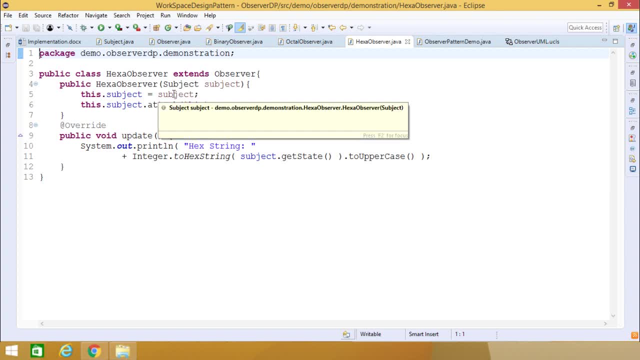 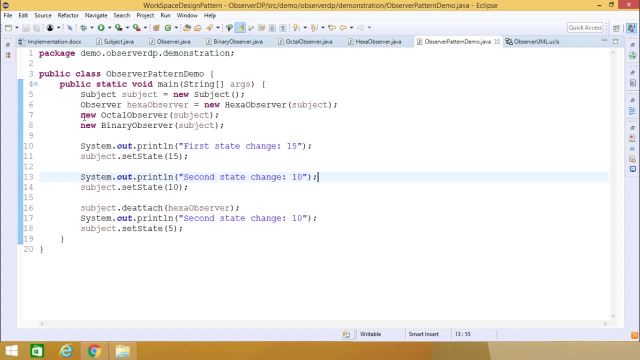 sub constructor, then this respective subject is getting instantiated and also it is getting attached with that array list automatically. similarly, we have defined to two anonymous, unnamed objects under the class octal observer and binary observer, passing this subject as input parameter. and now we are having this first state change is 15.. so we are going for subject dot set state 15.. so what will? 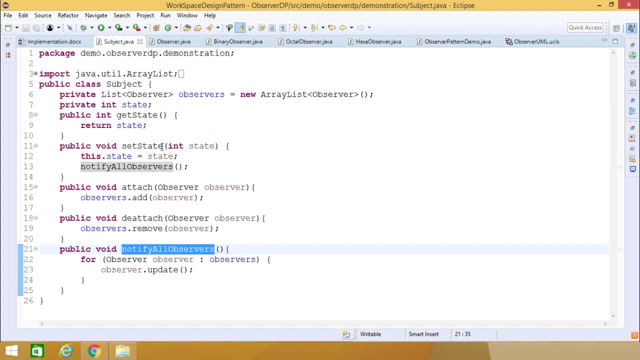 happen whenever we are going for, say, a set state, 15. 15 is the int value here. so notify, all observers will be called. this method will be called and this 15 will be kept in this particular state integer instance variable. so, in case of notify, we will be using this for loop and we will be executing the respective update function. 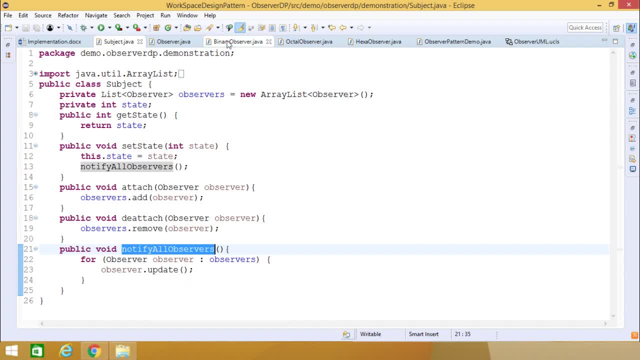 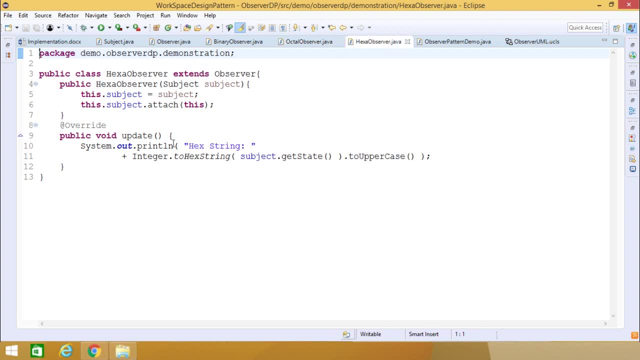 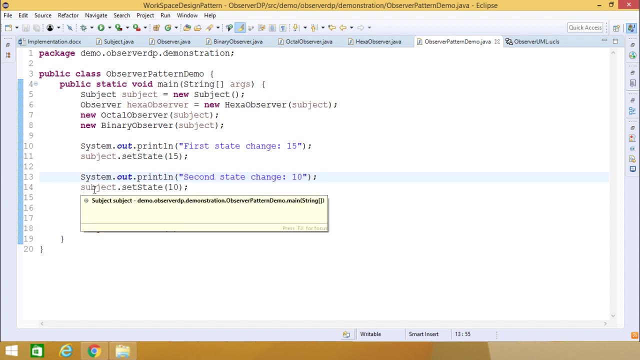 of the observer implementation. so now we are having this update function is like this. update function is like this because all of them are extending from this observer class update function is like this: so now again, we are going for second state change to 10. so subjects, subject, dot set, state 10: again, the updates will be called. now we are, we are detaching this, hexa. 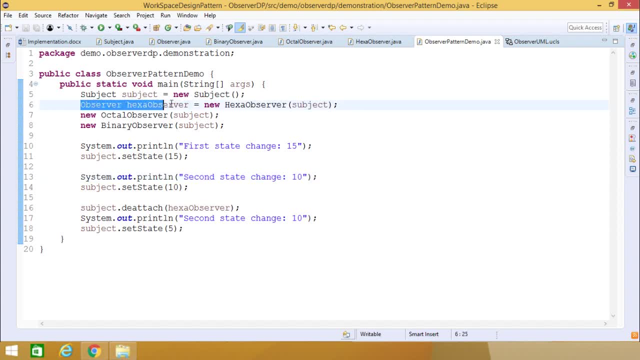 observer. so that's why here we have used some object name here, but for them, as I'm not going to detach them in future in this particular example, so I didn't go for any any object name here. we created anonymous objects dot detach. so this hexa observer has got unsubscribed. so now there is another change. 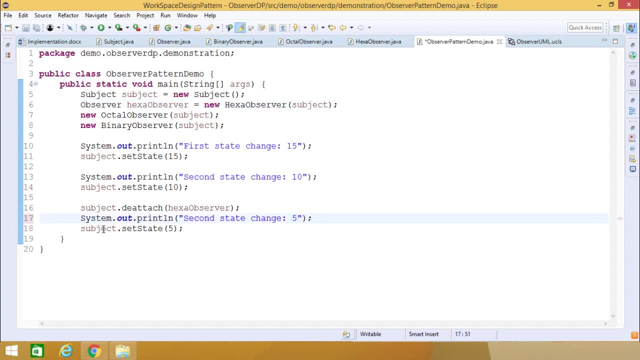 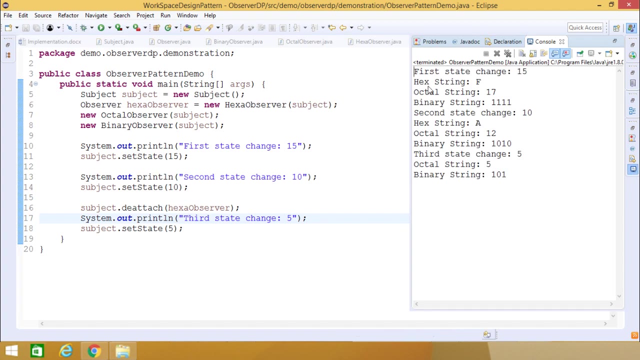 here. so I'm making this one. say five, say I'm making this one five. so subject: dot set state: we are having this five here. so what will happen? I'm making this one as third. so what will happen? let us see the outputs. so first change is the 15, so hex string F and octal string 17. why 17? 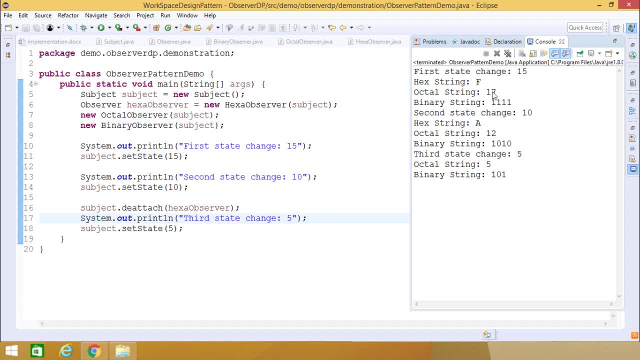 because 1 into 80 to the power of 1, that is 8, plus 7 into 80 to the power of 0, that is 7. so 8 plus 7, 15 will be there. so that's why it is 15, here it is F, here it is one seven. and here you. 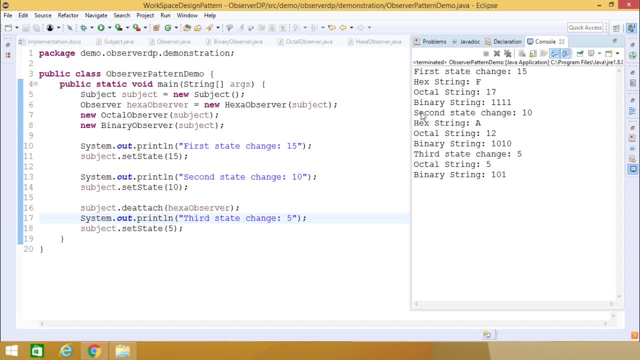 can find. in case of binary string it is one one, one one. now. second state change is 10 here. so hexa string is a octal string is 12, because 8 plus 2 is 10 and binary string is 1010. but in the last, 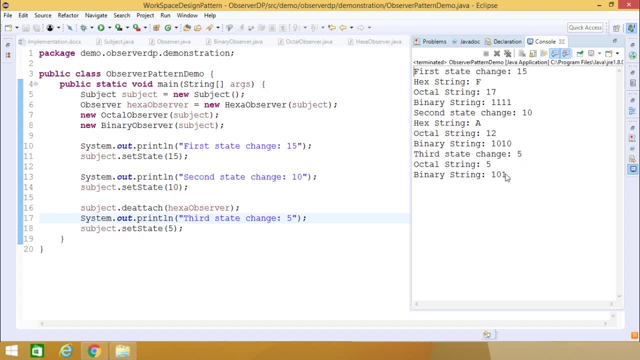 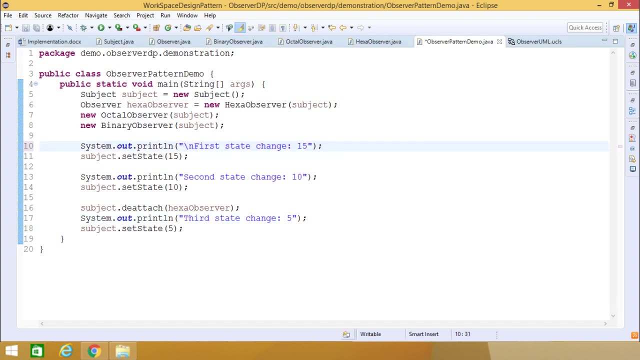 state change is 5, so octal string is 5, binary string is 101, but there is no hex string because it has got detached unsubscribed. before initiating this subject: dot set state 5.. so in this way we are getting this idea that how the things are taking shape. so for the better view, I'm just 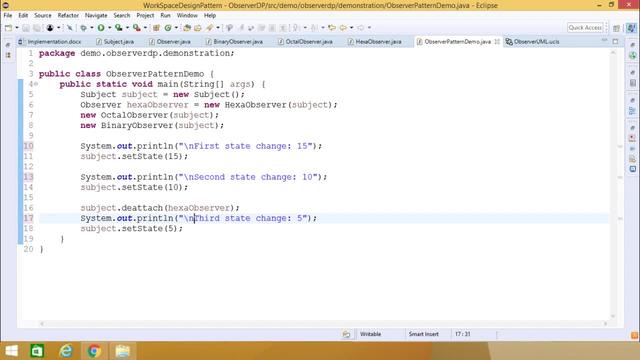 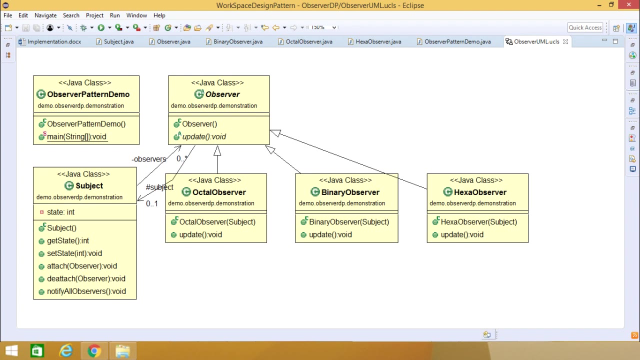 putting one slash in there. so now, if I execute, you can easily feel that how the things are taking shape. okay, now let us go for the class diagram. so here we are having this class diagram. so this is our Java class, that is the subject and this is our observer is there. so observer is abstract class. so that's why a is written. 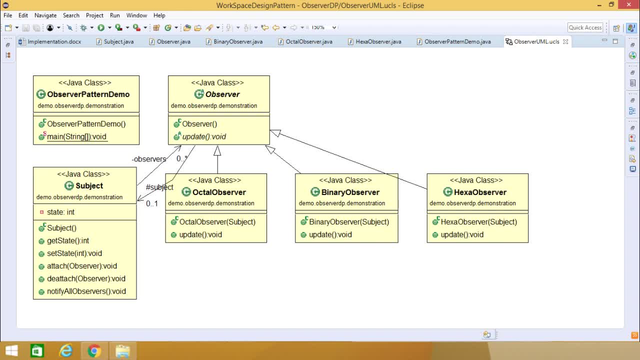 and it has got extended in the octal observer and then binary observer and then hexa observer and this particular subject is having observer objects, that is, the observers. observers, that is the under the private section. so that's why minus has come and it is a array list you can. 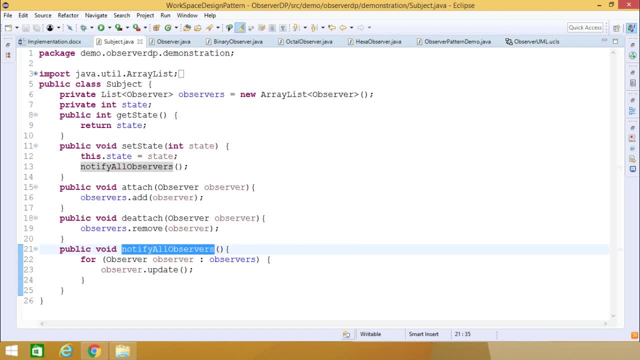 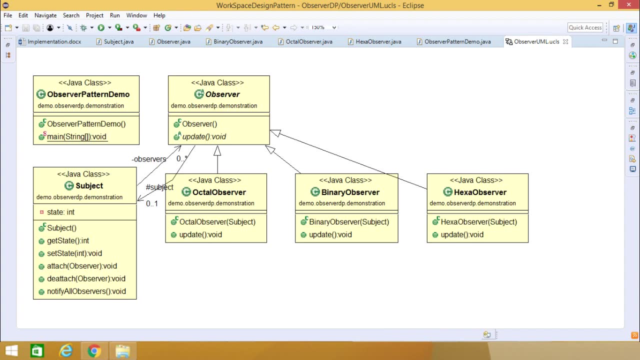 feel like find that to that one is subject. so it is under this private section. so list observer observes is equal to new add a list observer. so we are getting the same and now here, in case of, uh, in case of observer, we are having this subject. you can go to this observer.